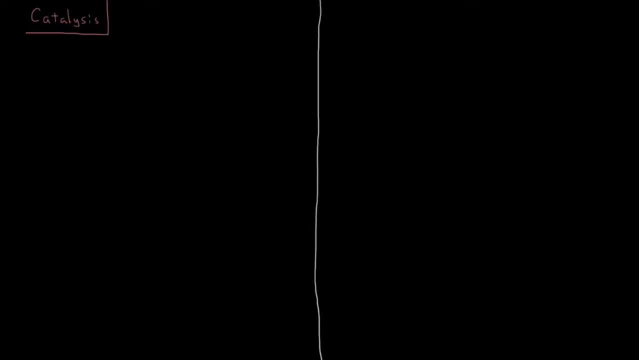 In this video we're going to talk about catalysis and how a catalyst affects the rate law and the overall rate for a reaction. So in normal reactions, as you increase the temperature, that means that you will increase the rate constant and thus you will increase the rate of the reaction at fixed concentration of all of your reactants. But it's not always available to you to go through that type of mechanism, because you can't always just increase the temperature. Maybe you have some other type of constraints which preclude you from increasing the temperature. Maybe your reaction occurs in some type of solvent which has a fixed boiling point. so you can't heat a solution past the boiling point, unless you get very clever with your experimental setup. But in any case, what you would want is some type of chemical species which can speed up your reaction at a reasonable temperature. So this would be. 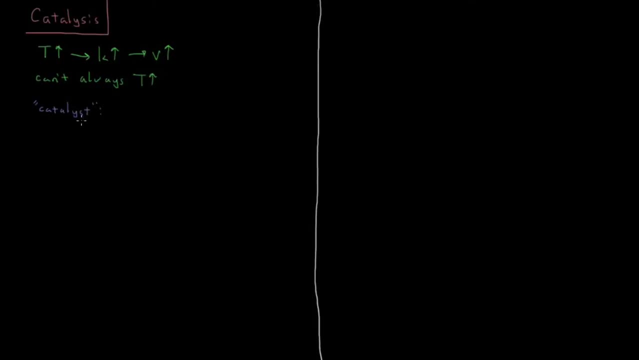 where the definition of a catalyst would come in. So a catalyst would be a chemical species that participates in a reaction without being consumed And hopefully, if it is a well-designed catalyst, it will greatly speed up that reaction. So a catalyst works by lowering the activation barrier. 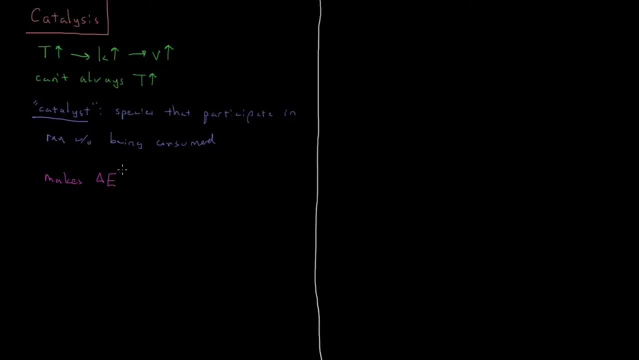 So in a video on kind of reaction coordinates and activation barriers. So a catalyst makes the energy change of activation much, much smaller And it doesn't change the equilibrium of the reaction. So it doesn't change any kind of. It doesn't change the enthalpy of reaction. 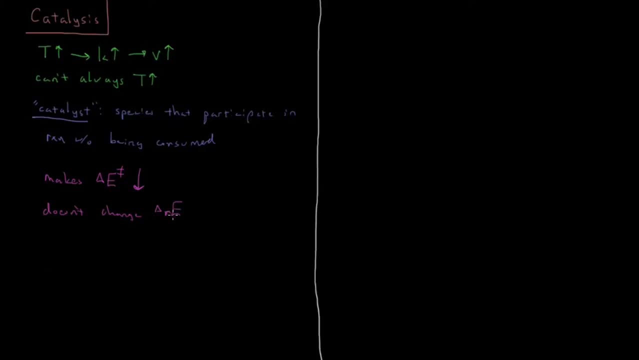 It doesn't change the Gibbs energy of reaction. It doesn't change any of the thermodynamics, It just changes the kinetics by making the activation barrier smaller. And so we can show this type of behavior by making a graph. So in this graph we'll have energy going up on our y-axis. 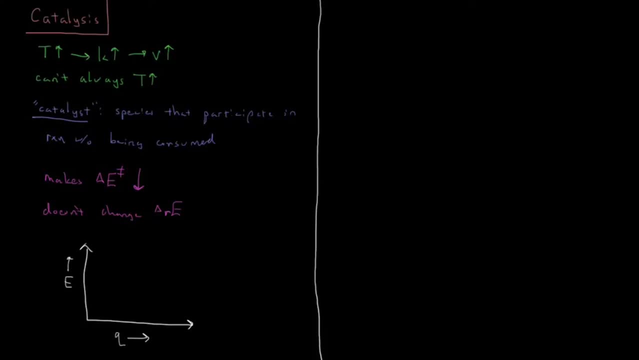 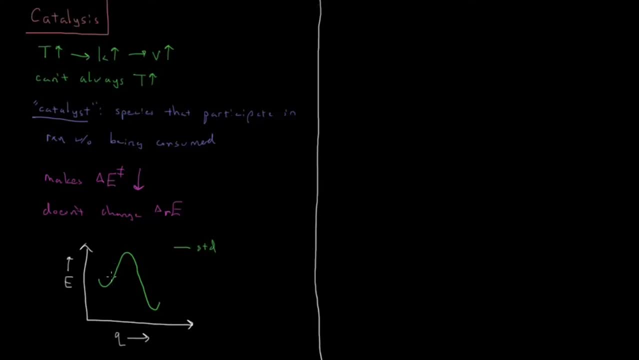 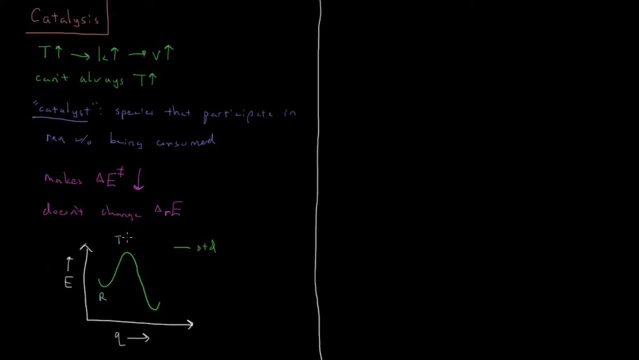 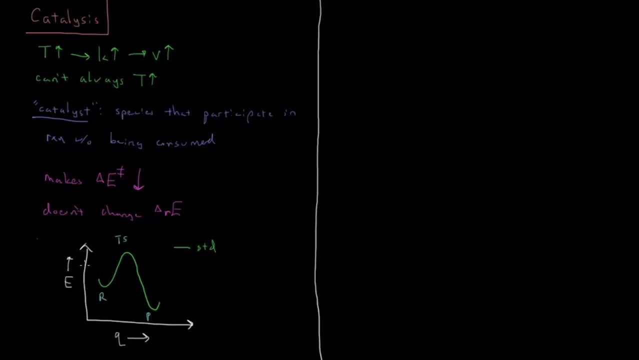 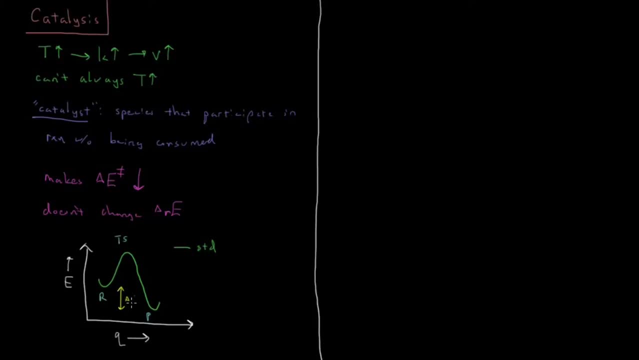 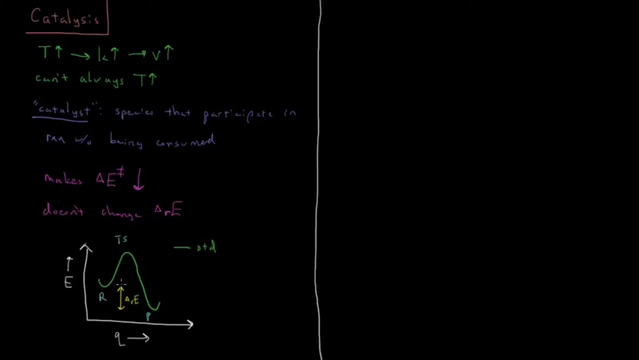 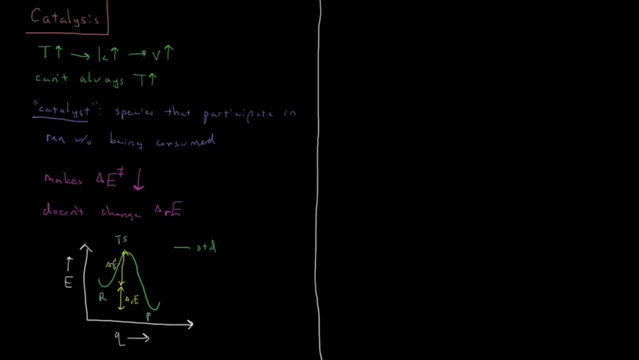 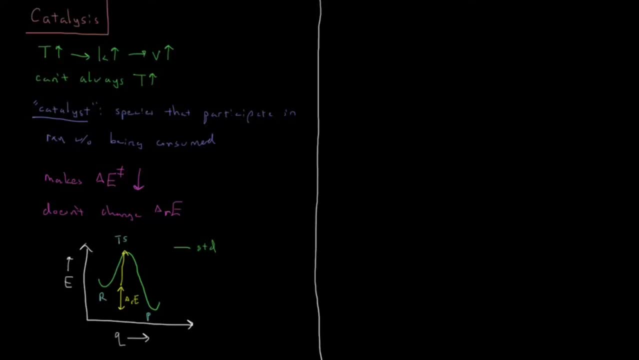 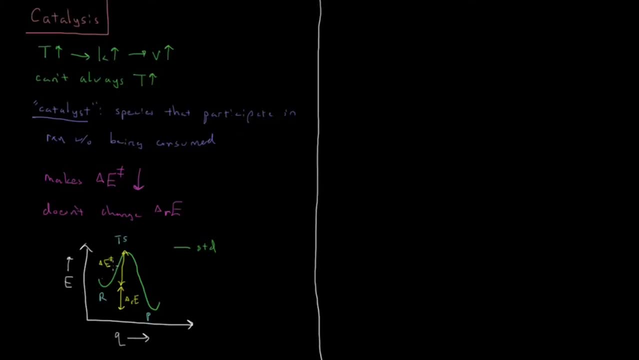 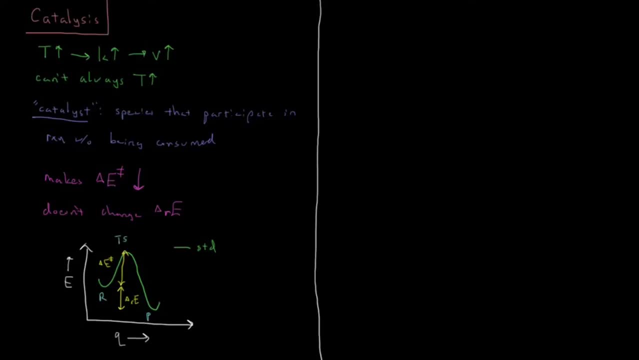 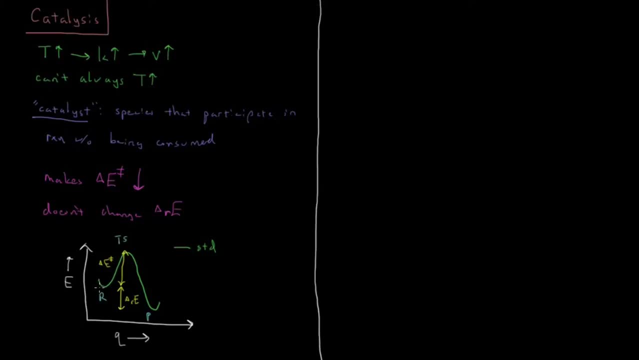 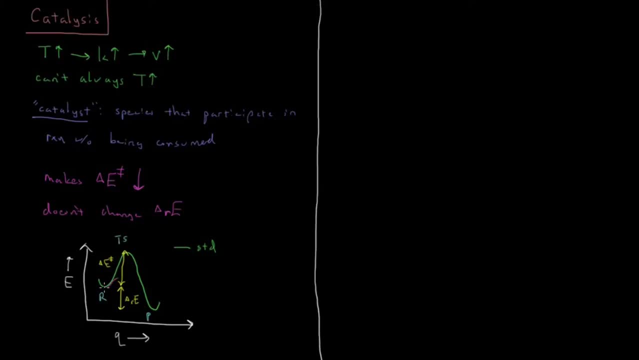 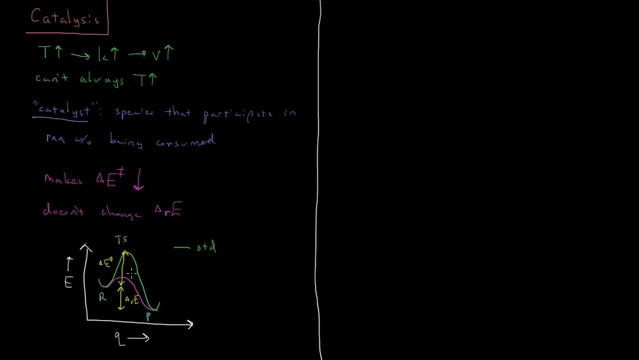 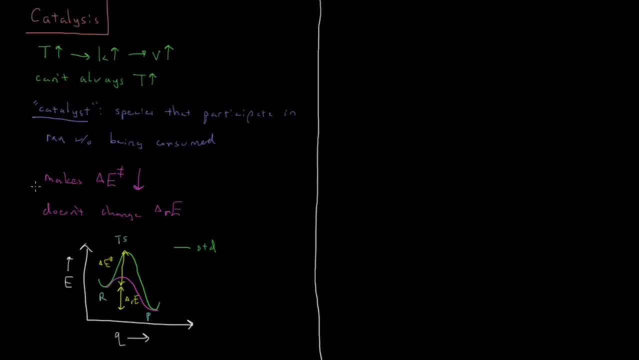 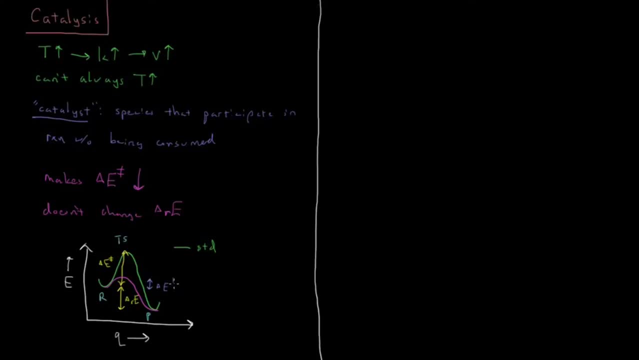 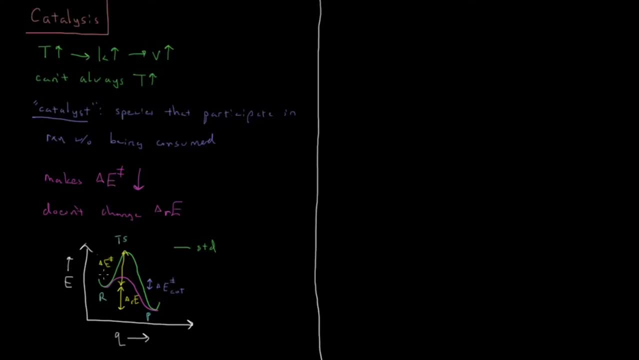 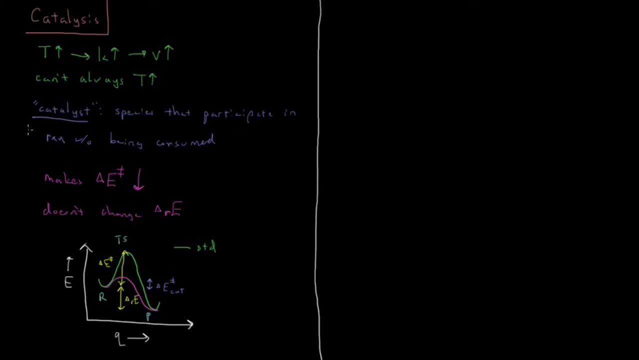 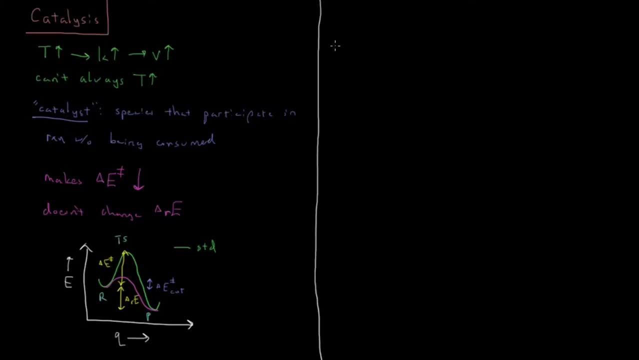 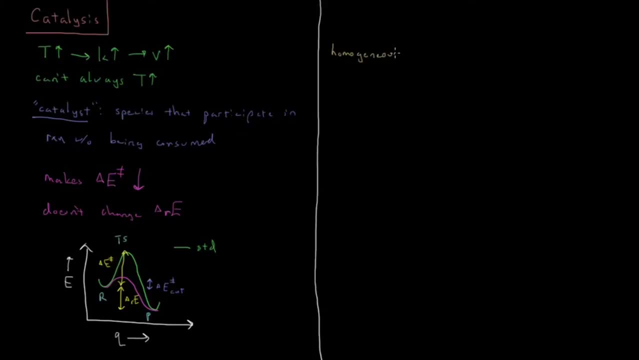 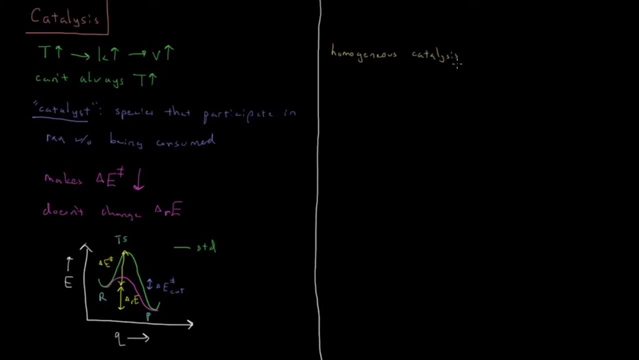 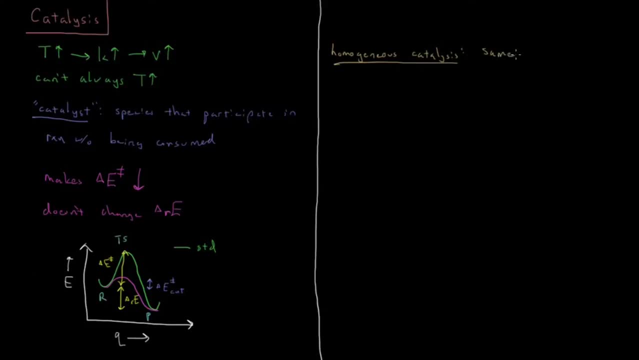 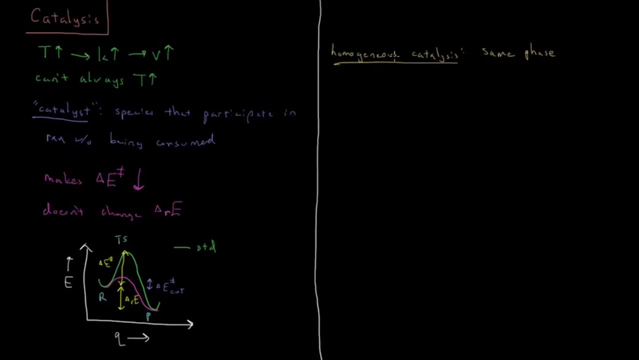 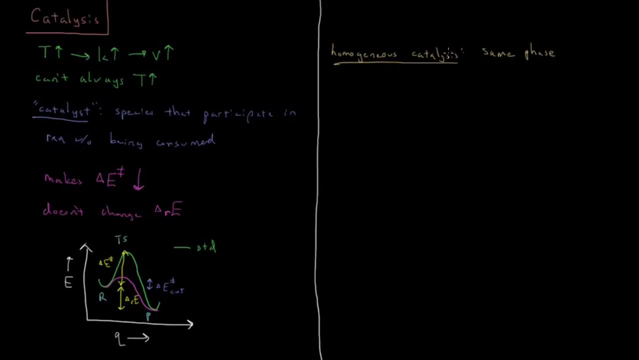 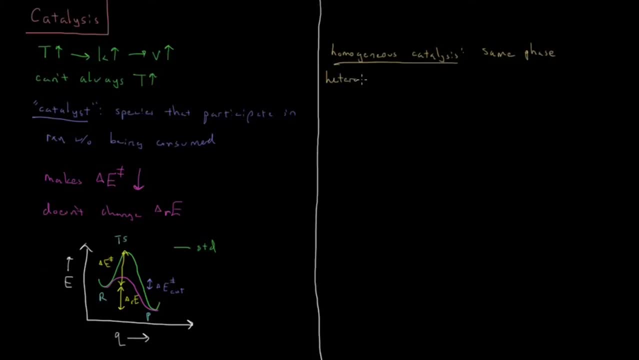 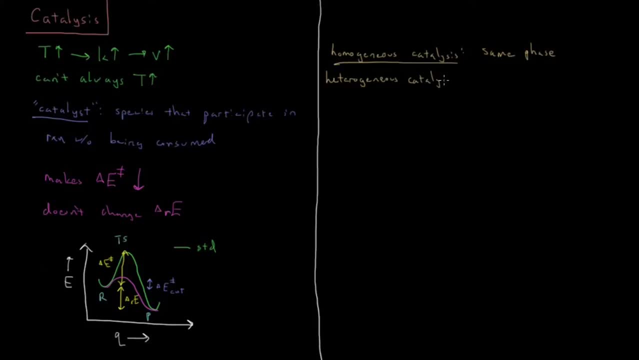 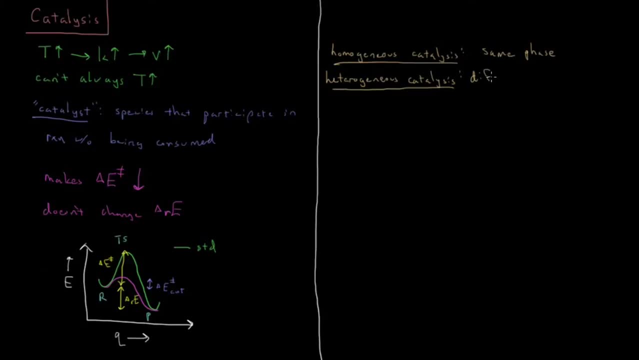 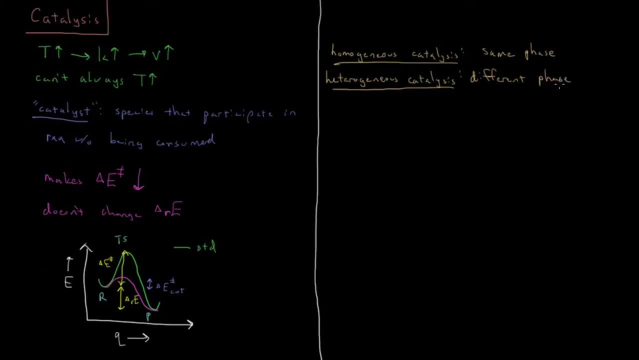 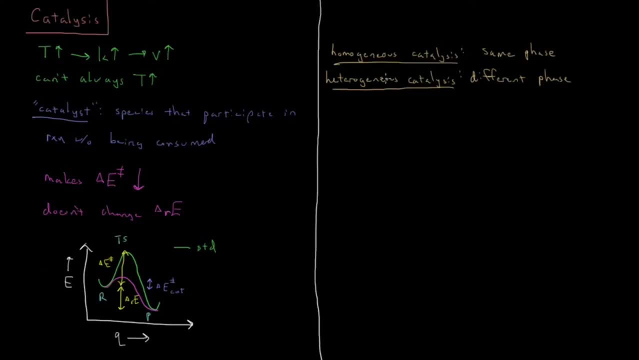 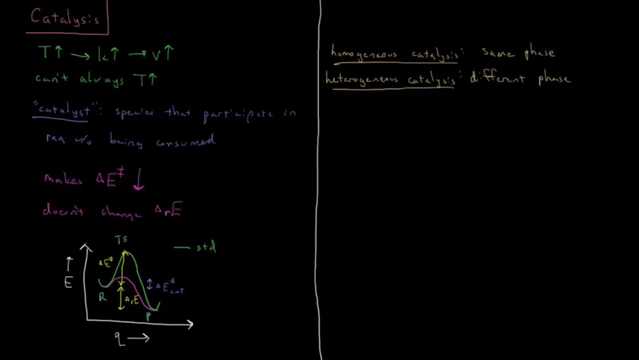 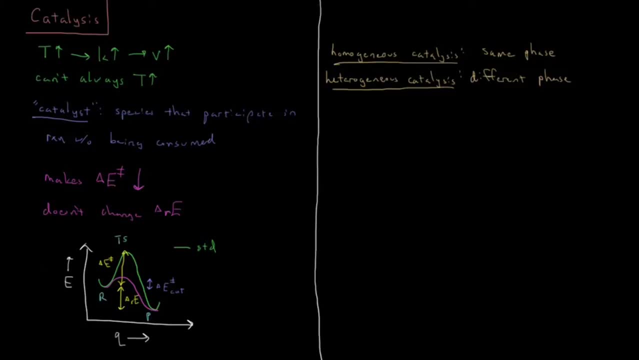 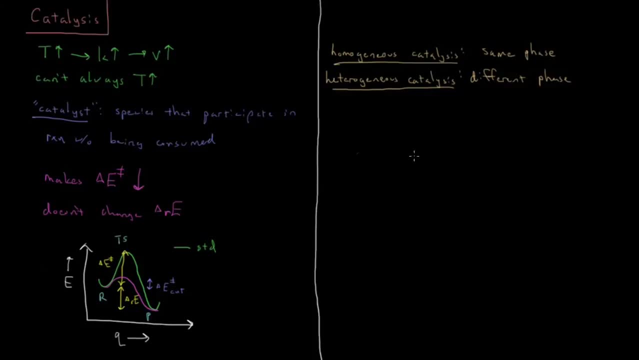 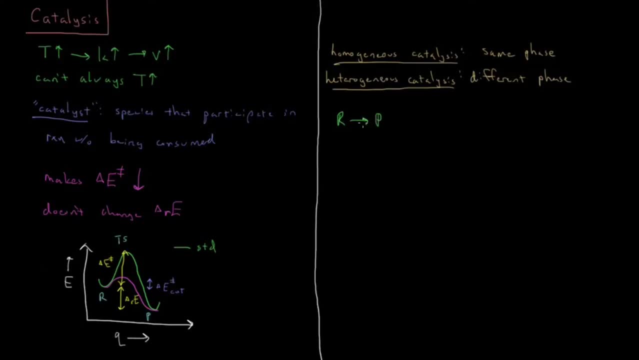 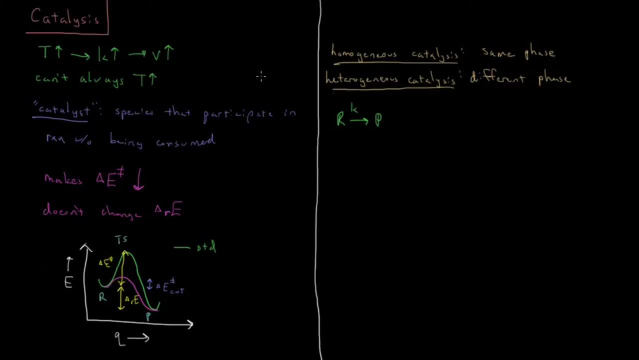 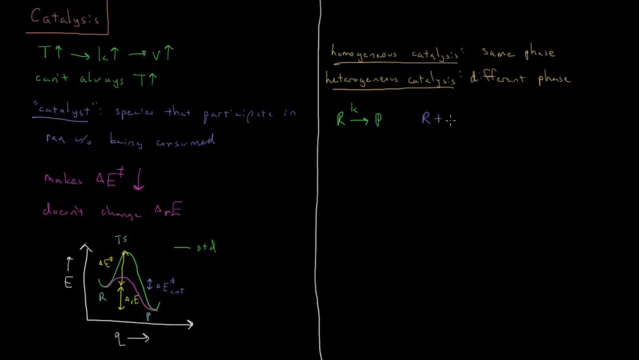 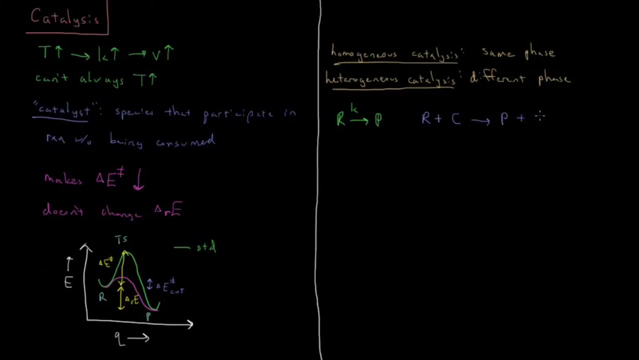 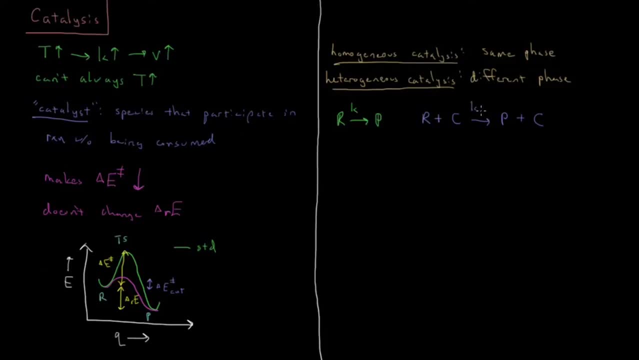 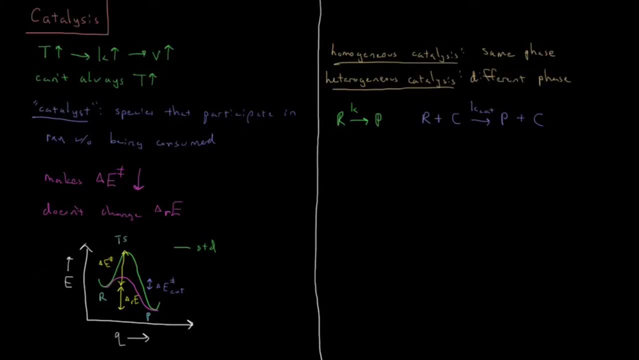 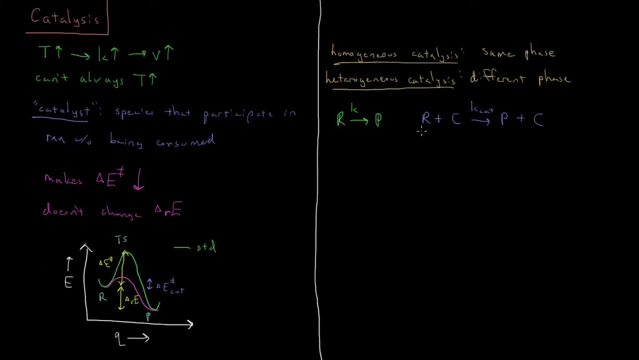 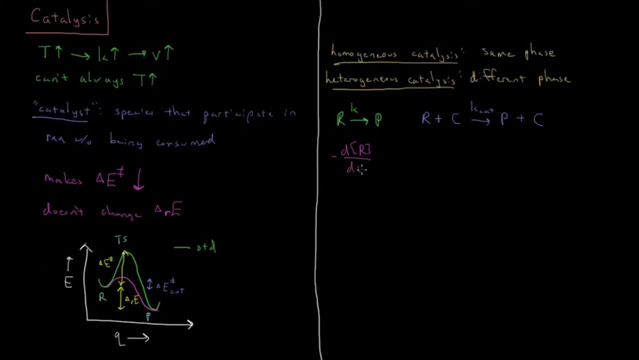 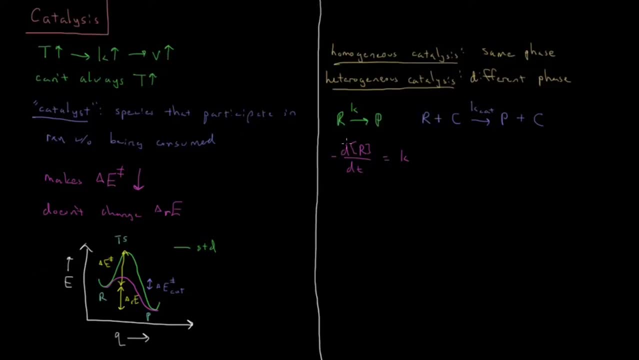 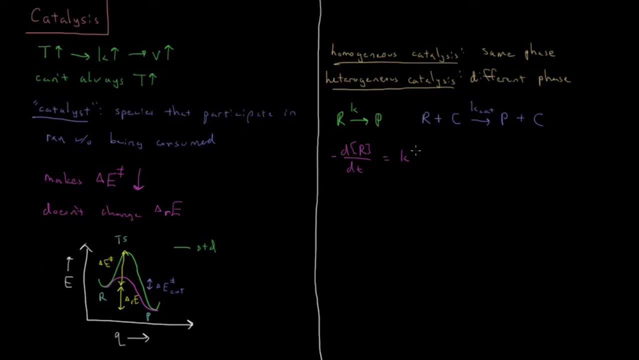 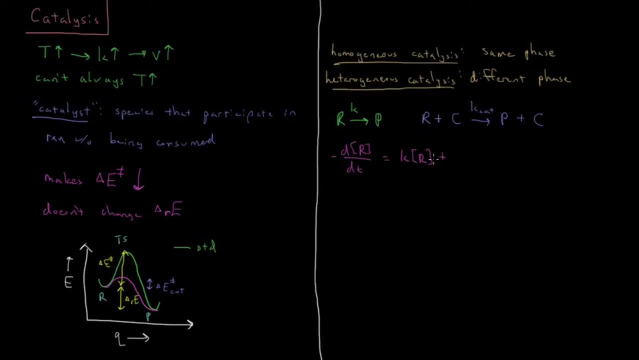 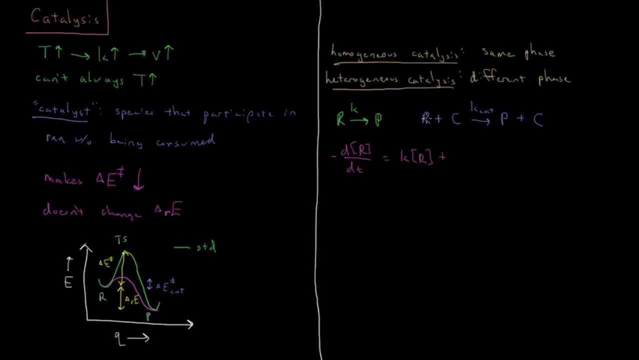 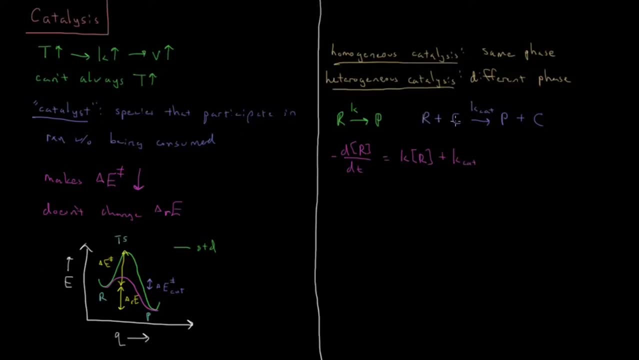 being second order. it's a reaction between the reactant and the catalyst. K cat times, R times C. okay, so can factor out, in this case, say dr dt equals, factor out the concentration of the reactant from it. so minus R. then in parentheses here we have K plus K cat times, concentration of catalyst. okay, so what? 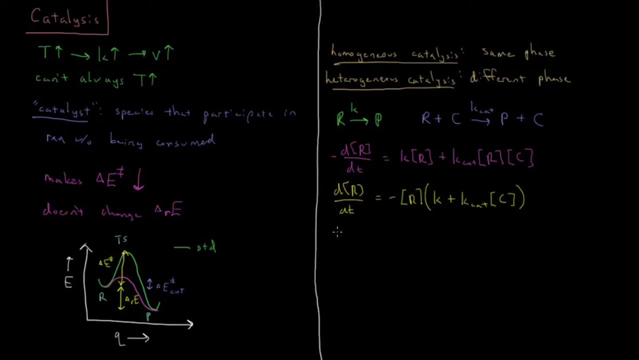 you see here is that in the, in the, even in the presence of a catalyst, your reaction is still first order in R. so it doesn't change the concentration dependence on R. generally what you have is K cat is much, much greater than K. so that is often the case, that K cat is much, much.